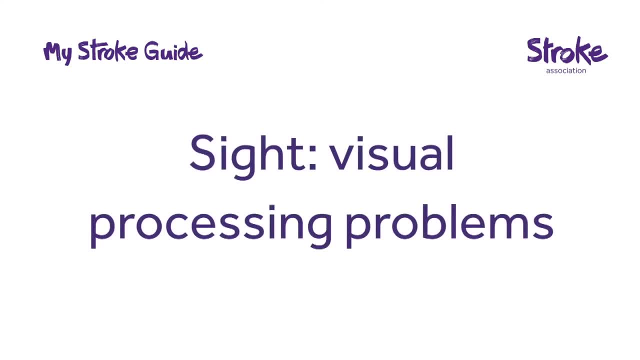 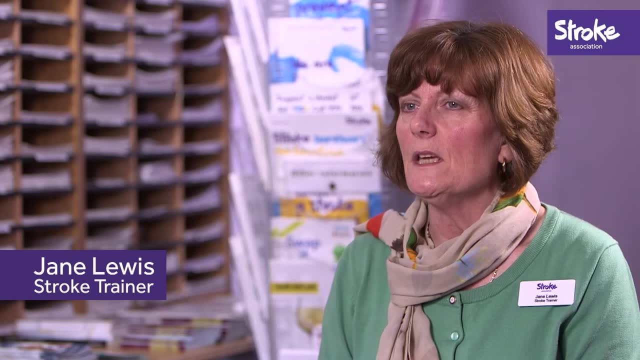 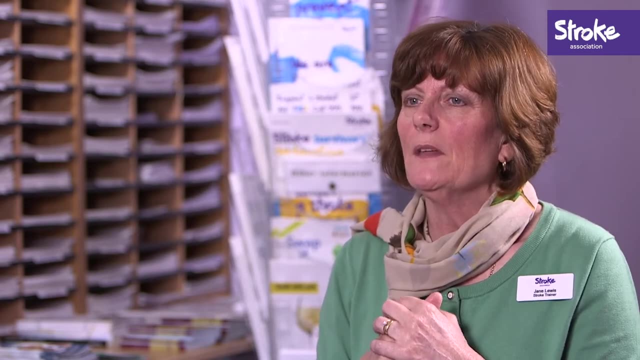 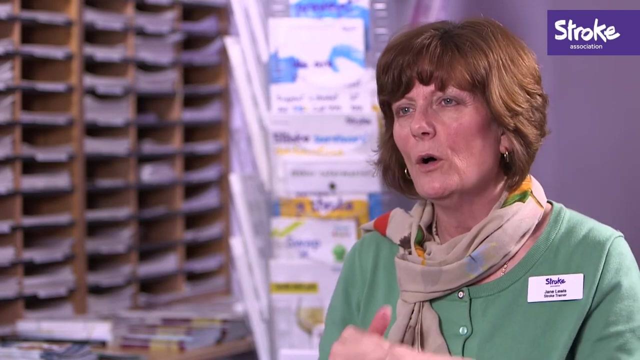 Visual processing is our brain's ability to make sense of and process the information that we see or take in through our eyes. and again, we do this in the occipital lobe of the brain. So we make sense of recognizing someone's face, we recognize an object, or we can pick out an object from quite 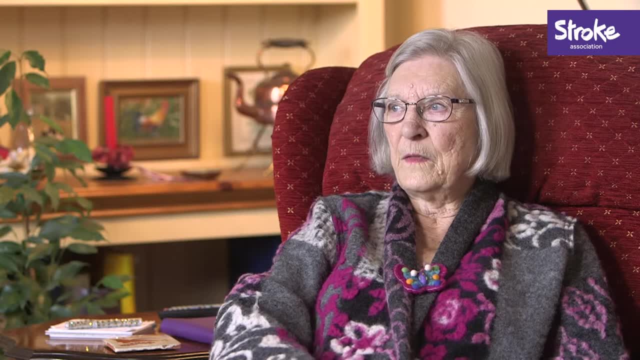 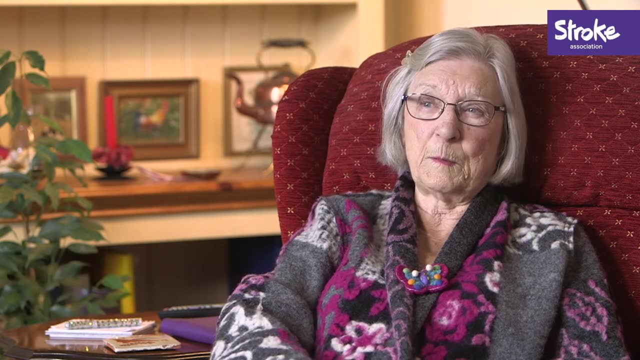 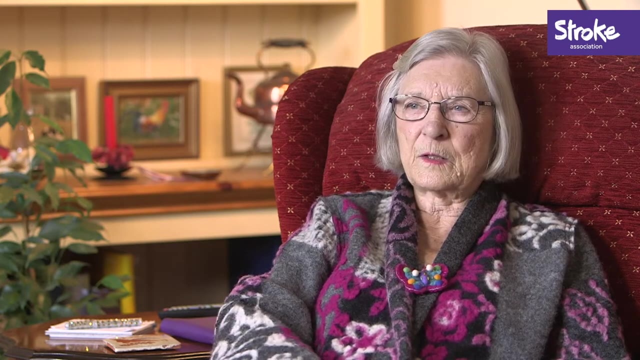 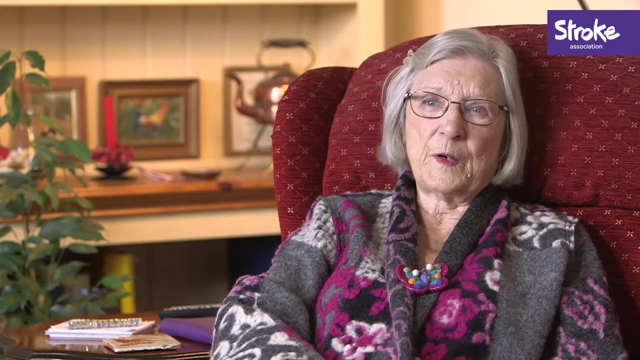 a cluttered tabletop, for example. Well, my vision after my stroke was practically non-existent. I couldn't see properly at all. so I had very heavy eyelids and so I kept my eyes shut most of the time, and when I did open them I couldn't focus on anything- The sorts of visual processing problems. 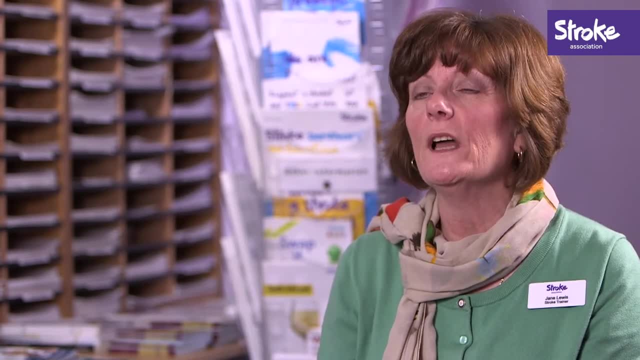 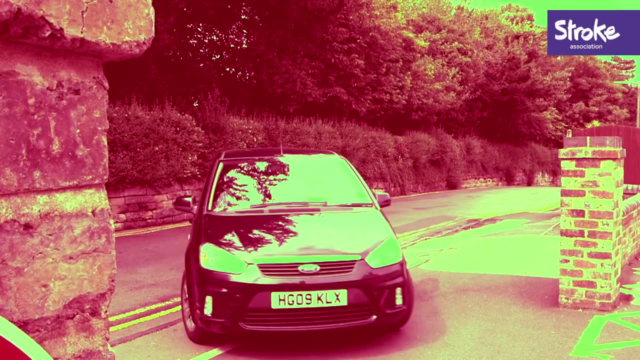 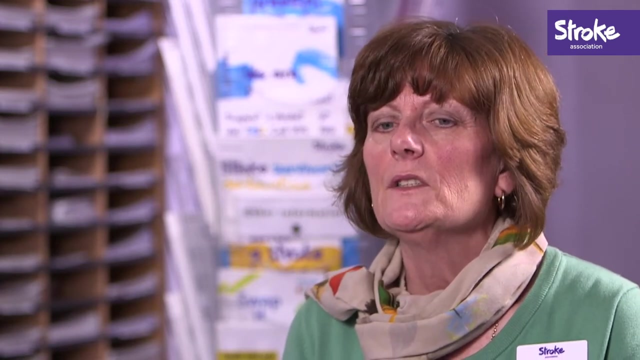 a stroke survivor might experience are difficulty with recognizing colors, difficulty recognizing faces, recognizing objects. sometimes they can't quite process them. Visual processing problems could be treated. depends on the individual, depends on the difficulties they're having. So if they're having difficulties with recognizing colors, for example, try and put a different color. 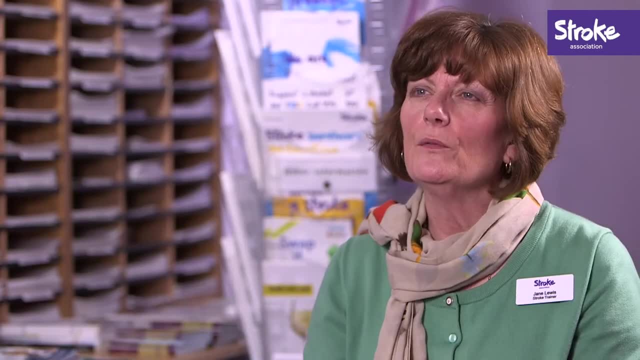 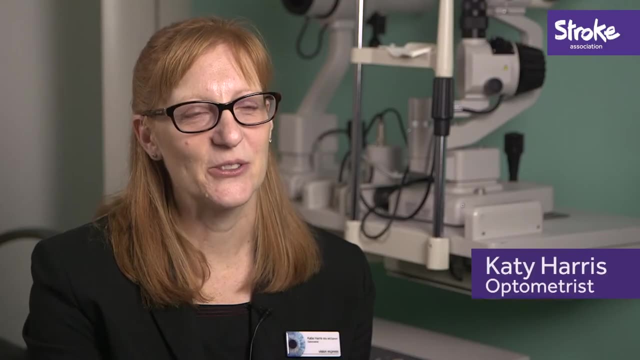 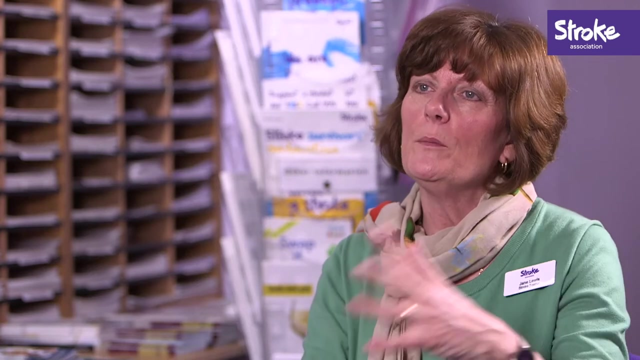 behind it. Think about contrast. They could have something called visual neglect, where they don't attend to one side of their body. Visual neglect isn't because you can't see something, it's because your brain can't interpret what you're seeing. And it could be further. it could. 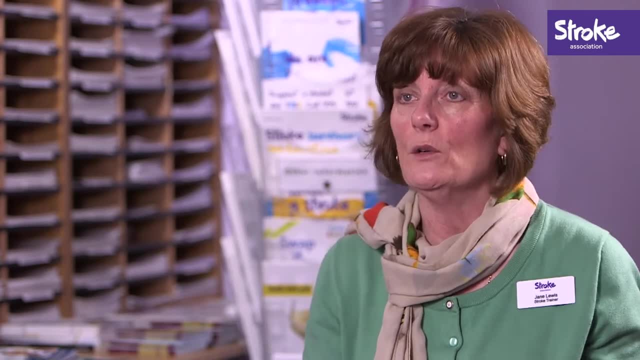 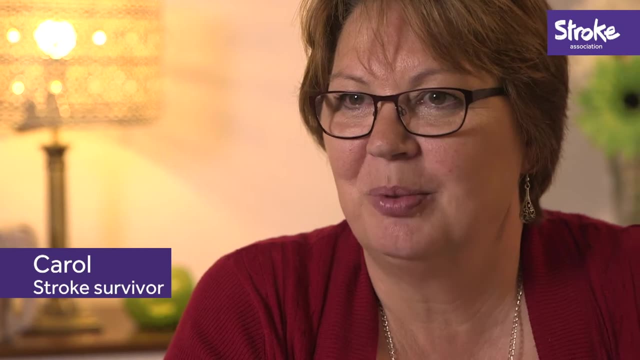 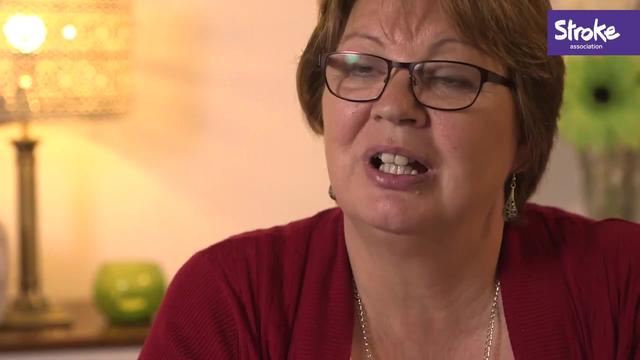 be wider so they might ignore the whole of space on one side or the other. Well, I should be really slim, really. you know, considering I don't see half of the food on the plate, I knock food off. you know, when I'm cutting, and that because I don't realize that there's food on the plate And you know if you. 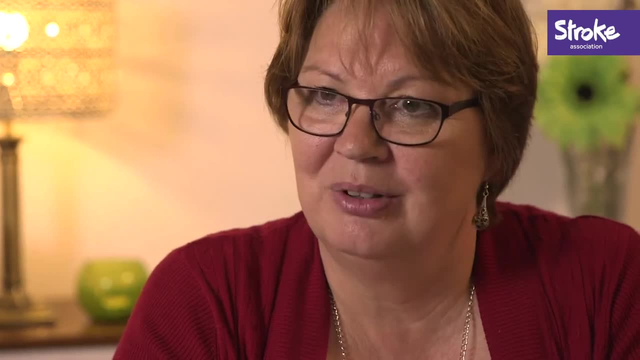 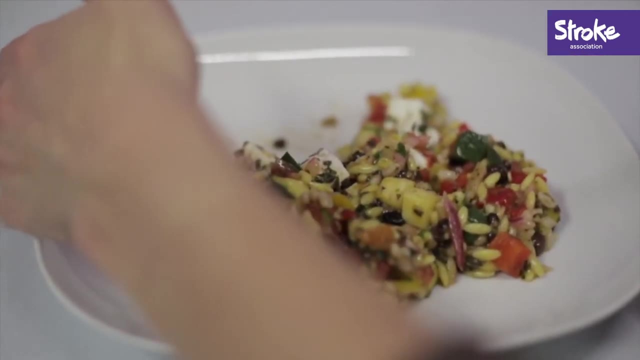 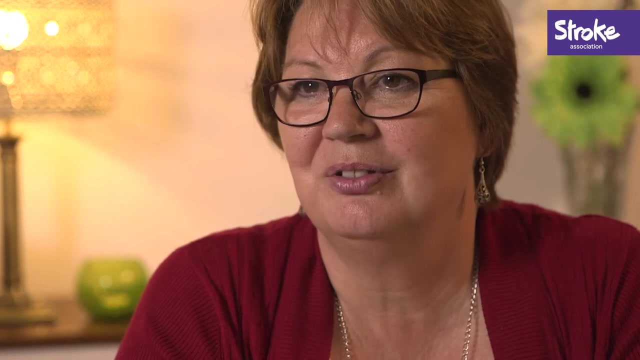 food there so it goes onto the table. I'm getting better now. I try to turn the plate so that you know I can see what else is there and you know. so it's sort of you know, keep moving the food onto the plate, So you do have to, sort of you know, think. 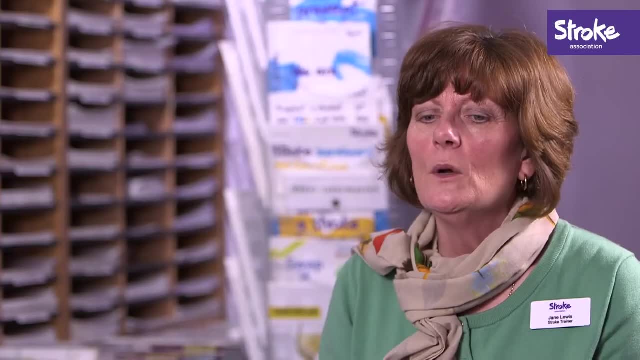 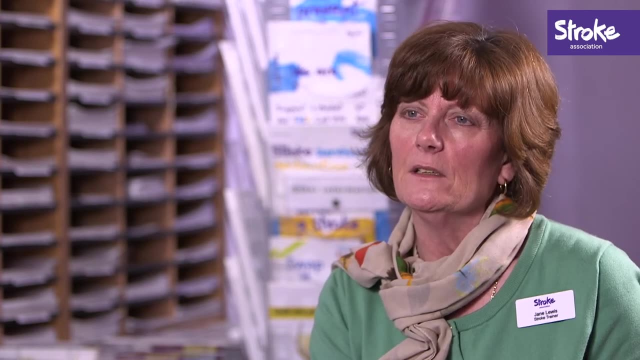 about everything that you do. You can't just take anything for granted With visual neglect. keep drawing the person's attention to the side that they are ignoring or they're neglecting. You know, really draw their attention, give massage, put jewellery. 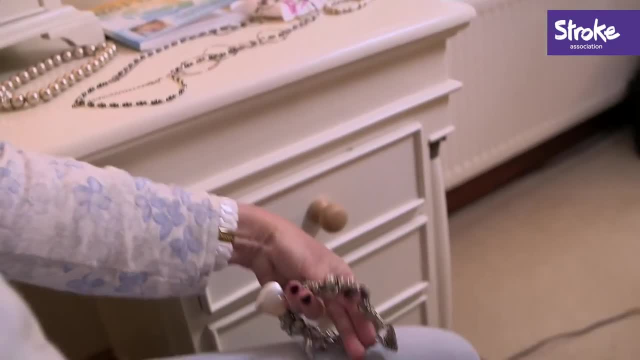 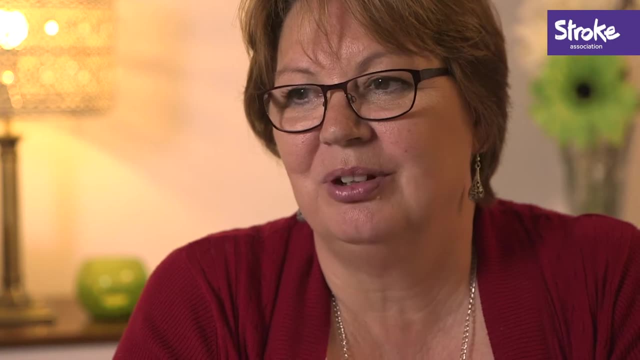 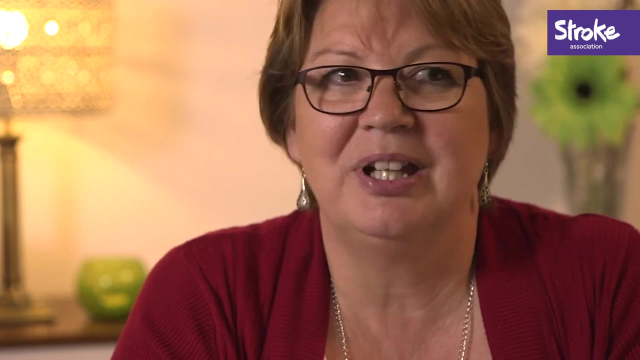 on that side or the side that's affected, to encourage them to use it and scan to that side in particular. It's hard, Shopping is hard. Whereas before you could look at something and see the whole picture, now you have to scan. you know you have to go along each shelf to look for something. 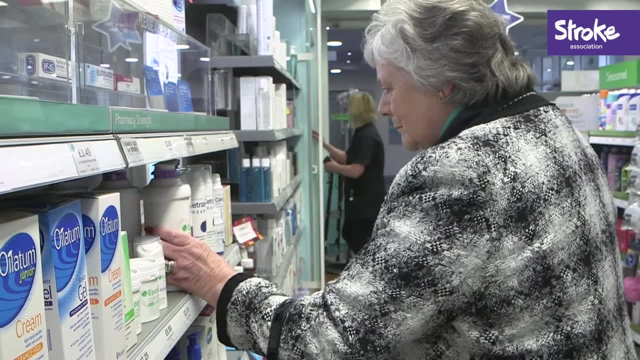 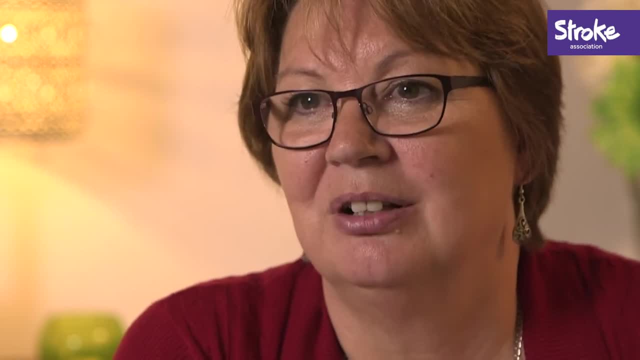 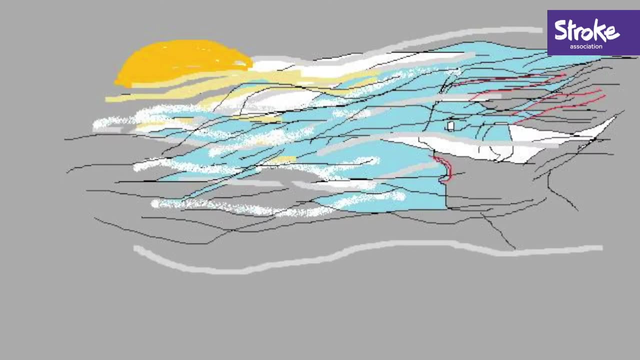 and shops are always moving things around, Yeah, Which makes shopping a real task. See, at a glance There is no glancing anymore, You just have to really concentrate and look. And another one is visual hallucinations. So people, or the brain rather, creates images. 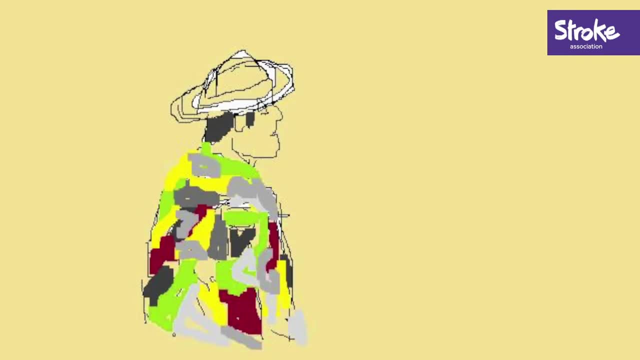 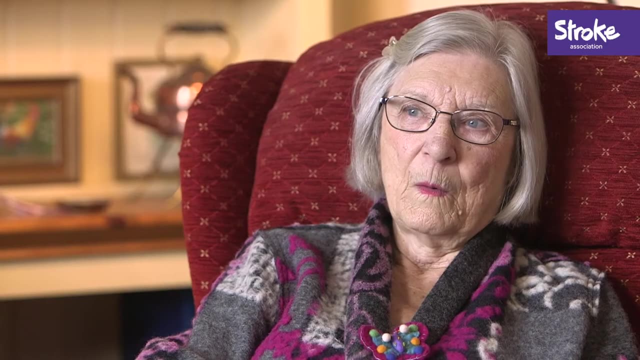 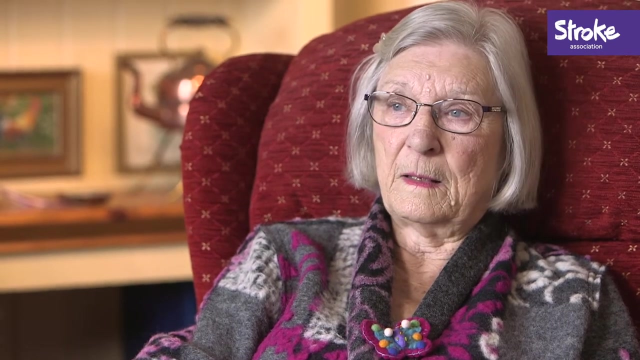 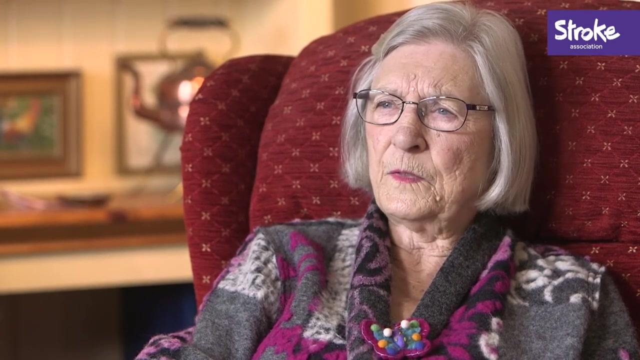 that aren't there. So they see scenes, complex scenes, or animals or people which they know aren't there. It can be quite disconcerting and worrying for people. Well, after my stroke I'd wake up. I'd wake up and see somebody standing by my bed, or I'd see a vase of flowers where I didn't. 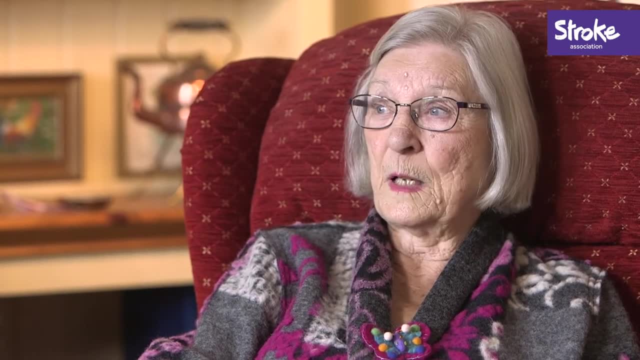 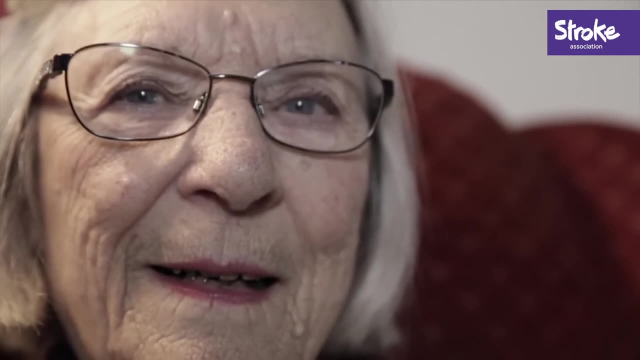 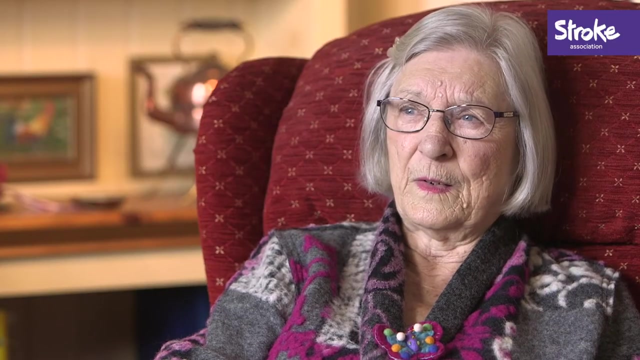 think there was a vase of flowers. Sometimes I'd be looking at the television and I'd see a whole lot of action going on behind it and think, well, is that part of the programme? In fact, so many different things that I made drawings of them all because I found it so. 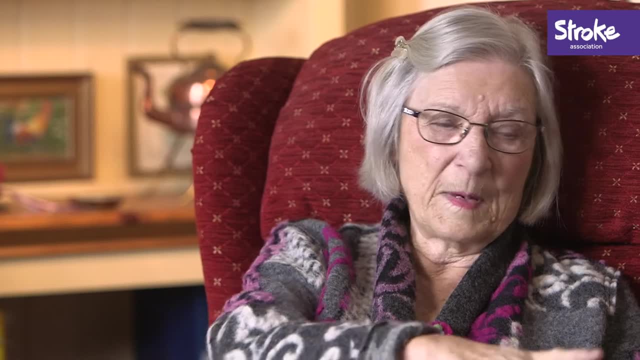 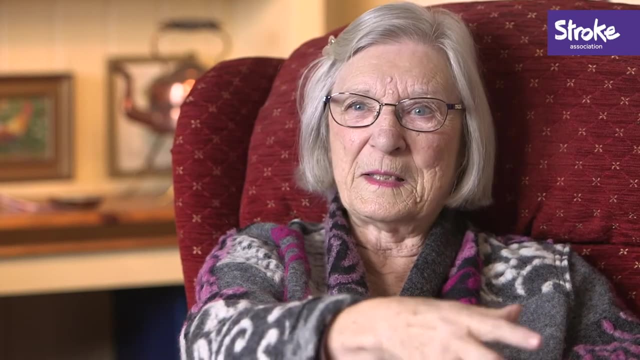 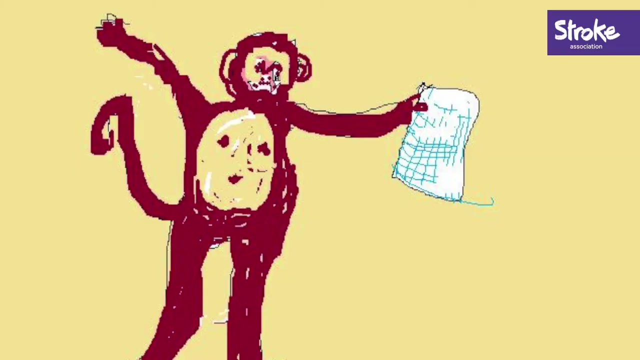 fascinating. Like some. a monkey would come into the room holding something and I'd get up to go and see what it was and they'd just disappear And all kinds of really interesting things. I told the specialist about it. After a while she wrote to my GP and said: well,